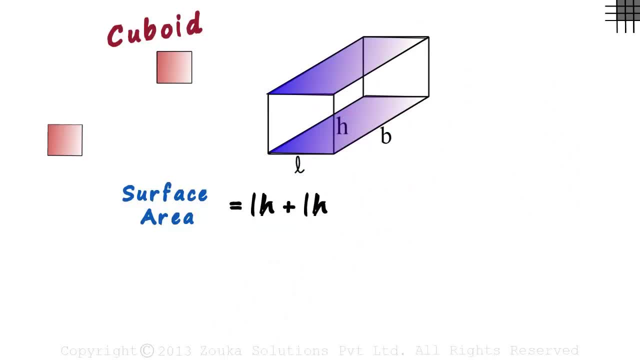 The area of the rectangle on top will also be the same as that of the bottom. Their sum will be LB plus LB. Now let us take these two to the side. We have covered front and back, top and bottom. What remains is the side faces. 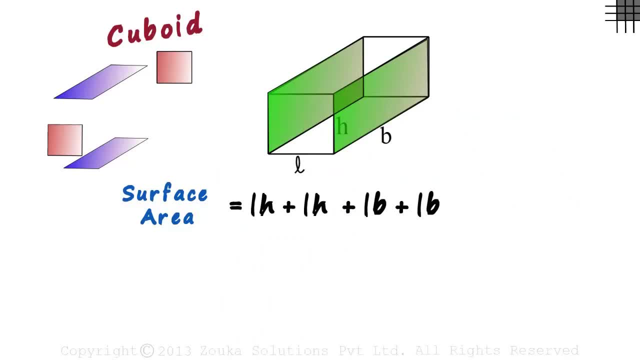 The sum of the areas of the rectangles at the sides will be BH plus BH. Area of each rectangle is base multiplied by height. Look at each group. This will be 2LH, this will be 2LB and this will be 2BH. 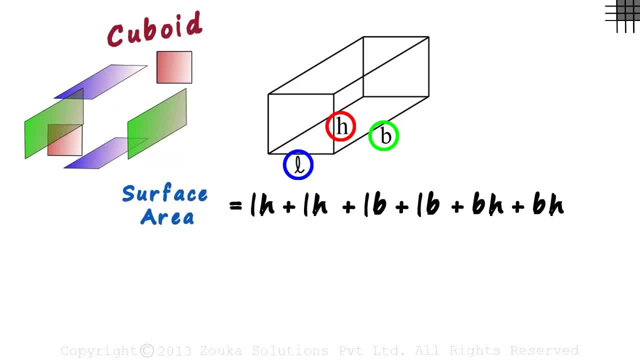 So for a cuboid with L, B and H as dimensions, the surface area will equal 2LH plus 2LB plus 2BH. As 2 is a common factor to all the terms, we write it as 2 multiplied by LH plus LB plus BH. 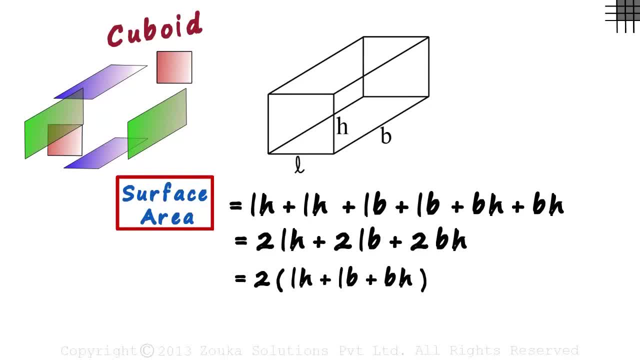 That's how simple the concept of surface area is. We just need to look at each surface individually and add their surface areas. Within surface area there is a concept of lateral surface area. Remember one simple thing: Lateral means side, So this would actually mean. 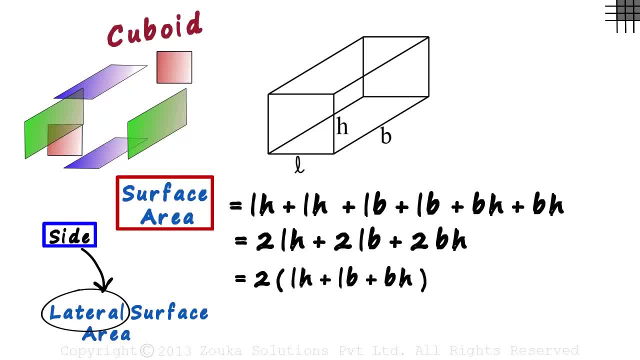 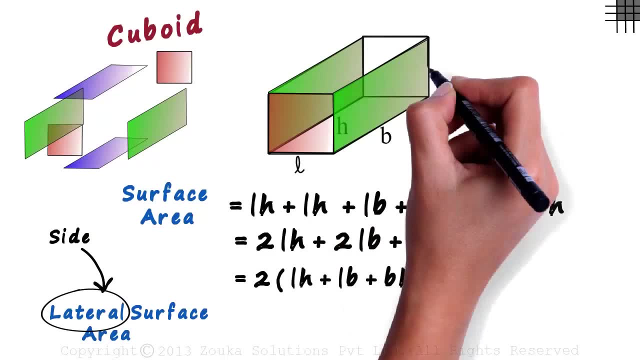 the surface area of rectangles at the sides. There are four such rectangles: This one, this one, this one and the one at the back. In terms of surface area, you can also look at lateral as everything except the top and the bottom. 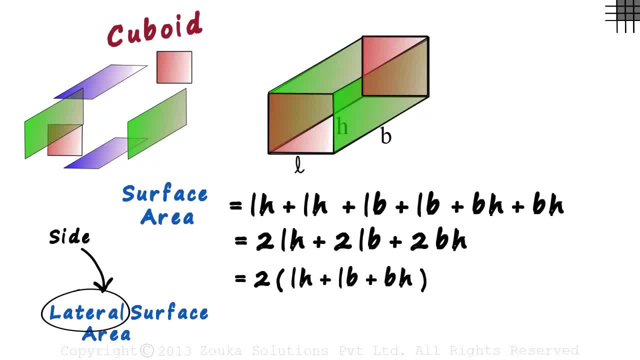 The two green and the two red rectangles make up the lateral surface. The lateral surface area just equals the sum of the areas of these four rectangles. The sum of the green rectangles would be BH plus BH and the sum of the red rectangles will be LH plus LH. 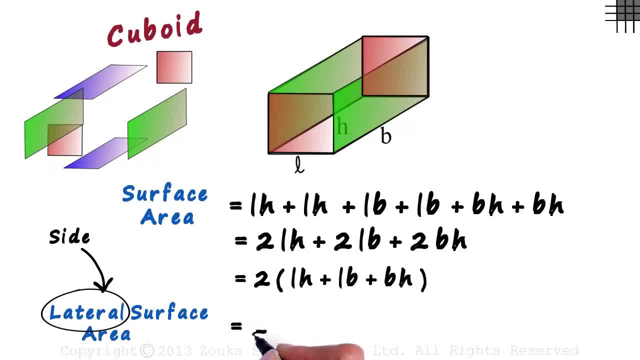 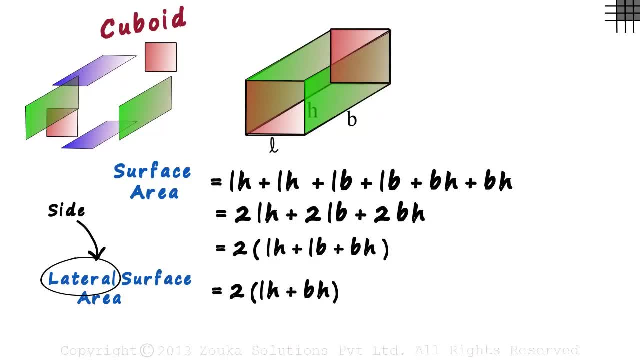 The total lateral surface area will be twice LH plus BH. Where do we use this concept of lateral surface area? Well, here's one of the applications If you want the exterior of your house painted. you do not paint all surfaces, You just paint the sides.